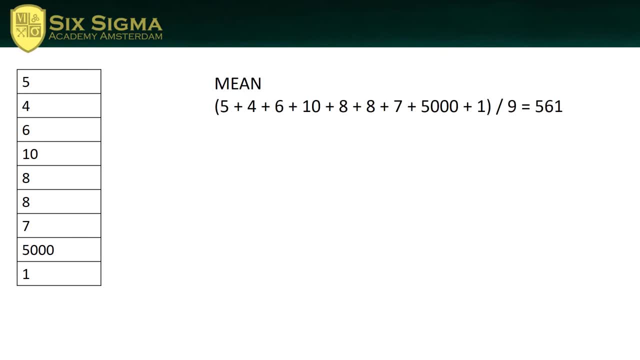 Now, if you want to calculate the mean or average, this is what we should do: Add these values up, which is what we did here. Divide them by the number of observations. We have nine players, We have data about nine players, So we have nine observations. So we divide everything by nine, which means that, on average, the player spent $561.. The mean is 561.. 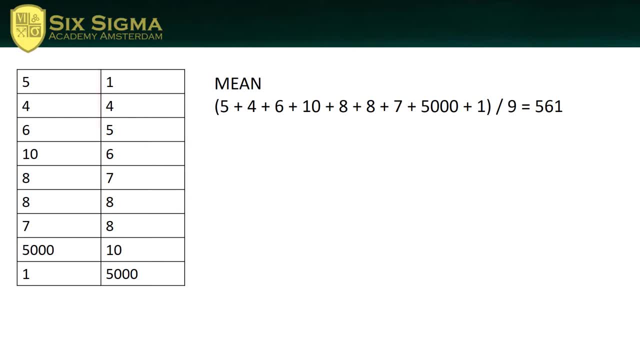 Now let's calculate the median. In order to calculate the median, let's calculate the median. In order to do that, we have to order the data from low to high, And then the middle value would be the median. Well, in this case, the middle value would be seven. Okay, So that would be the median. 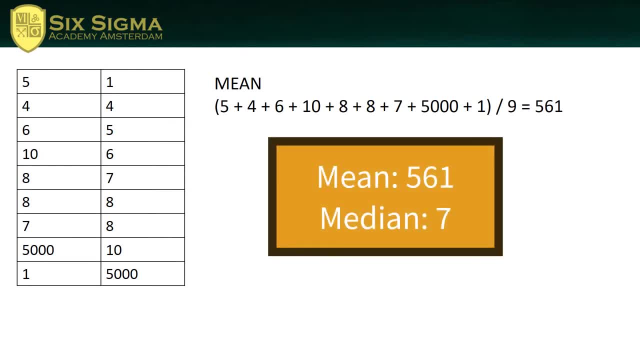 Now let's compare the median and the mean, Both of them measures of central tendency. There's a big difference between them. What is causing that big difference? The big difference is caused by the fact that the mean is much more sensitive to extreme values than the median- Much more sensitive And it is much more influenced by the 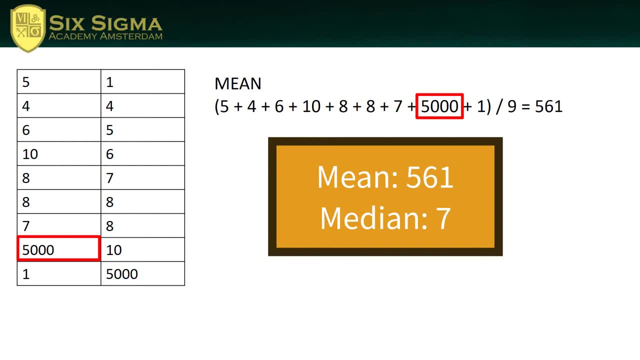 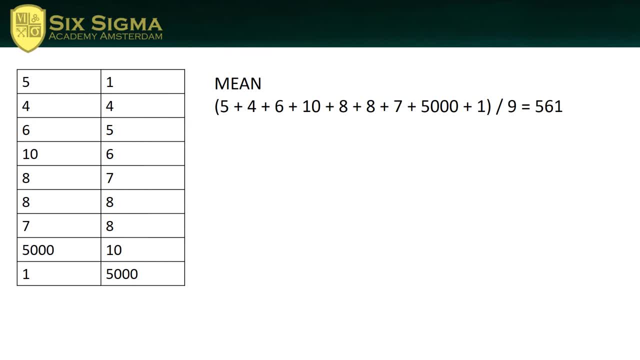 investigate, I would quickly see that, hey, what is causing that is this 5,000.. Then you have to take another important decision. Once you found out that the 5,000 is indeed causing this- and it is an extreme value- you have to decide: do I eliminate the 5,000 or not? Do not eliminate it. 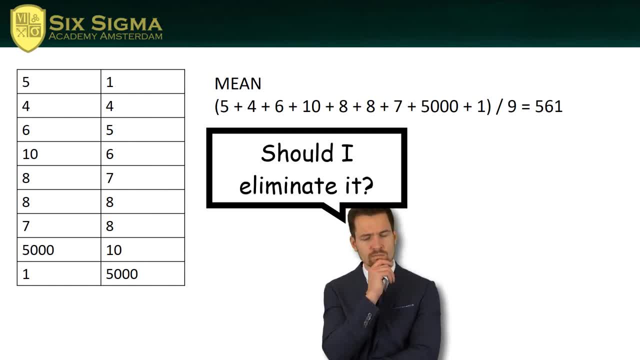 if it is just part of your data. If we have here a group of nine people, if every group of nine people, or many groups of nine people, contain one person such as this person, a person who is heavily addicted, who cannot control himself or herself and spends incredible amounts of money, then this